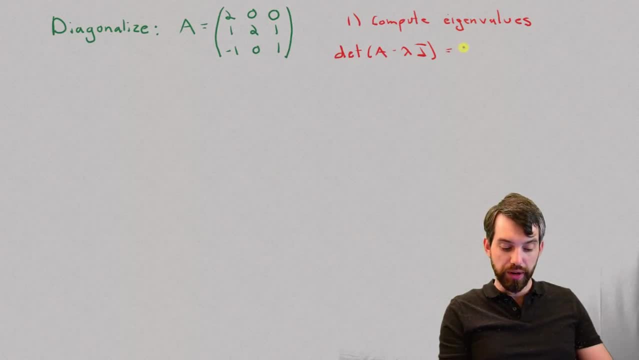 And the question is: when is this determinant going to be equal to zero? That will give me my eigenvalues. So I'm going to use a vertical line for computing the determinant. I'm taking: 2 minus lambda 0, 0, 1, another 2 minus lambda a, 1, and minus 1, 0, 1 minus lambda. 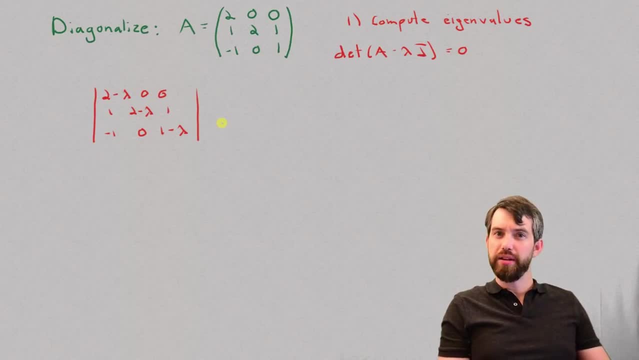 Because I have these zeros on the top row. when I compute the determinant and I expand along the top row, two of the terms are just going to be zero, And the only one that's really interesting is the final term. So this is the 2 minus lambda term, And then it's multiplied to the determinant. 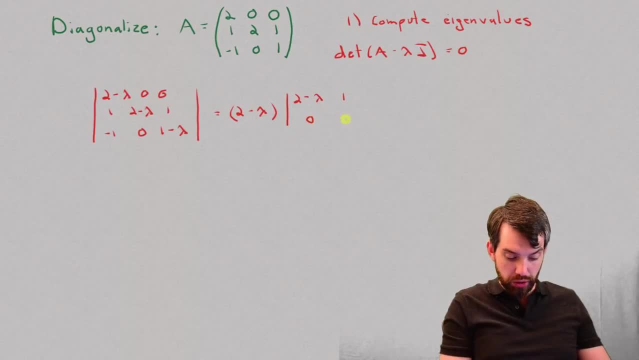 of 2 minus lambda, 1, 0, 1 minus lambda. In other words, I'm looking down here at this submatrix here, So, continuing on, I can compute that, Fair enough, it turns out to be an upper triangular matrix. 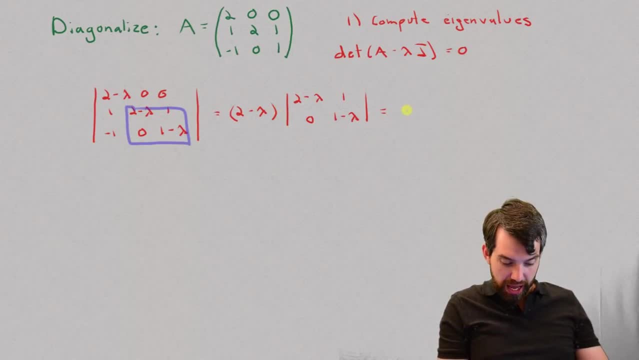 and so it's going to just be the product of the diagonals. In other words, I'm going to have 2 minus lambda with algebraic multiplicity 2.. I'm going to put the squared up there And then, finally, multiplied by 1 minus lambda, I'm setting that equal to zero. 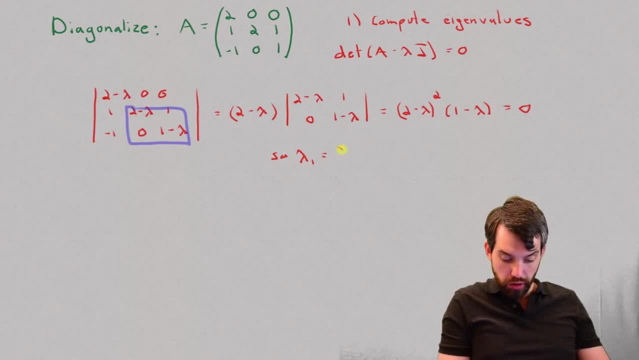 And so I get that a lambda 1 is equal to 2.. And then I get a lambda 2 is equal to 1.. I notice that lambda 1 is going to occur twice. All right, so now let's continue and move on to step 2,. 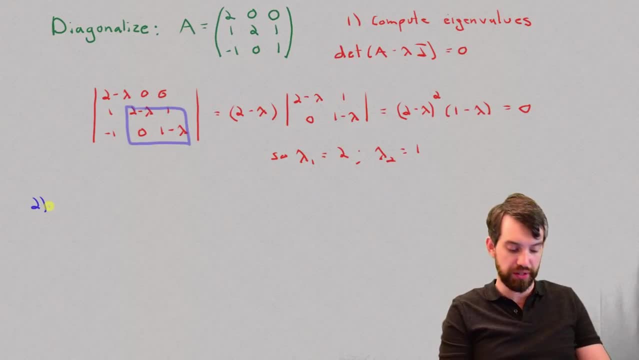 which is computing the corresponding eigenvectors. So I'm going to do the lambda 1 equal to 2 case first, And therefore I am investigating the a minus lambda i. That matrix, when multiplied to x, is going to be 2 minus 2 is a zero. Then I have another. 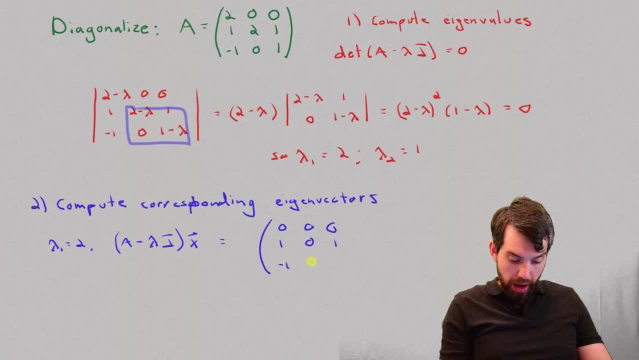 minus 2, so another zero here, And then minus 1, 0, minus 1.. And then I'm trying to solve this system being equal to zero and asking what vectors of x is going to have this property. Well, it looks like I can do a little bit of a reduction to the matrix. 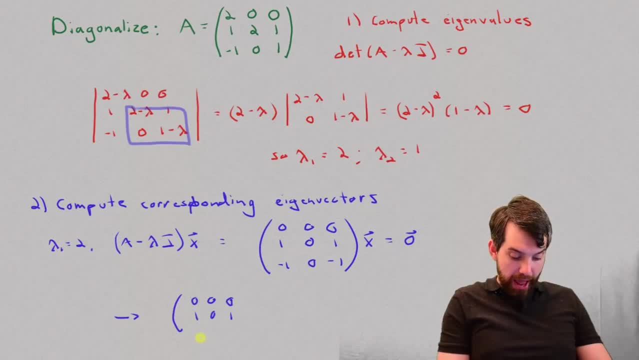 0, 0, 1,, 0, 1, and then I'm going to put a row of zeros down here, because it's just a multiple. The third row is a multiple of the second row, And then, if I want to solve this particular system, I note that I have two different free. 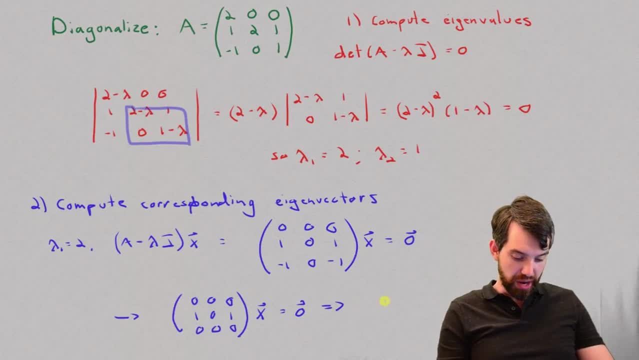 variables. So my x2 and my x3 are going to be free, And so let's put those in. x2 is an s, x3 is a t, And then the only equation I really have to look at is this second row here, the only. 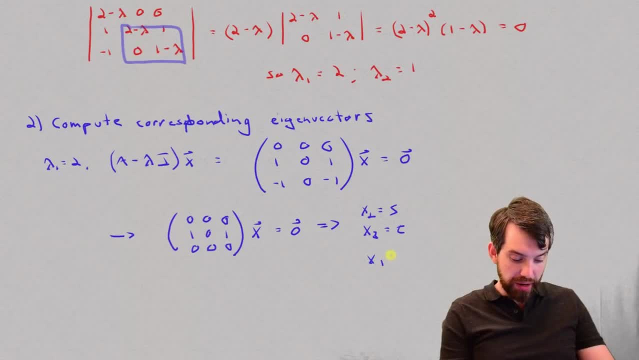 one that's trivial, And it tells me that my x1 is going to be equal to minus the x3, in other words minus t. So the canonical way that we want to write down these solutions to homogeneous systems is to say: look, it's going to be the scalar s times in x1. there's no s's, so it's 0,. 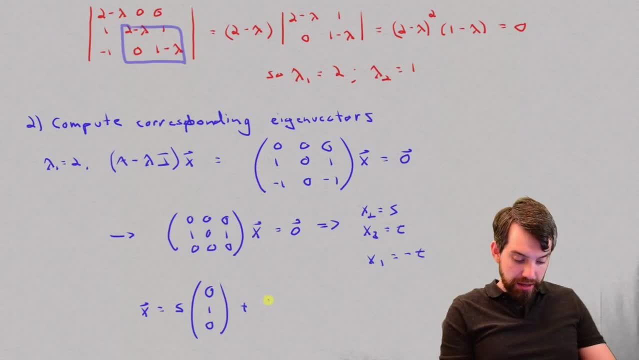 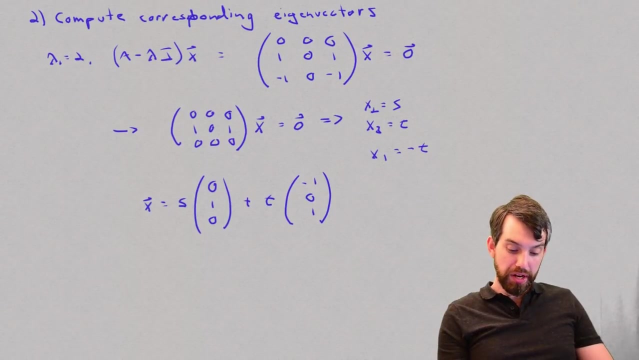 and then 1 and 0. And times t and in x1 I have a minus 1, a 0, and a 1.. So that's our sort of standard way to write down the solutions to this homogeneous system. Now I want to note here that we've got these two vectors. 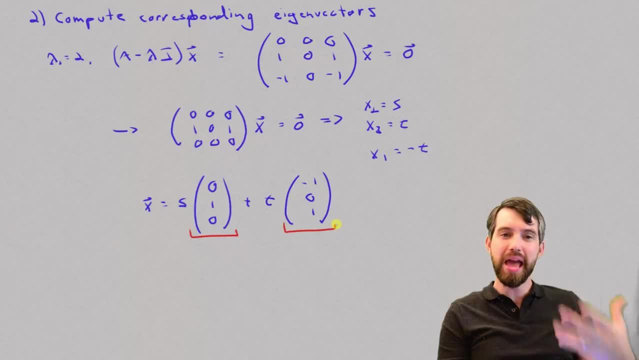 And you'll recall, when it gets to diagonalization, the demand was for this matrix P, who's going to have columns? that were the eigenvectors. the eigenvectors had to be linearly independent. But we've previously argued that when we go through the Gaussian algorithm and we get 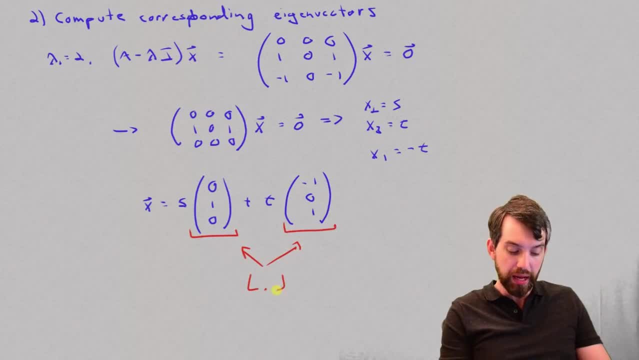 these two different vectors here, that they are going to be linearly independent. indeed, That's what the Gaussian algorithm is always going to deliver, And so it's going to be very good that we have these two linearly independent eigenvectors corresponding to that same eigenvalue that had algebraic multiplicity too. 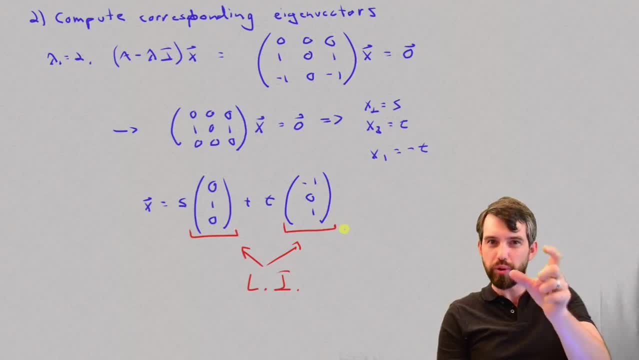 So there is lambda, There's lambda, There's lambda of equal to 2, that that was repeated twice, but that we also got two linearly independent eigenvectors. We're going to need that to be the case, So this is a great result for us hoping to be able to diagonalize, and we'll come back. 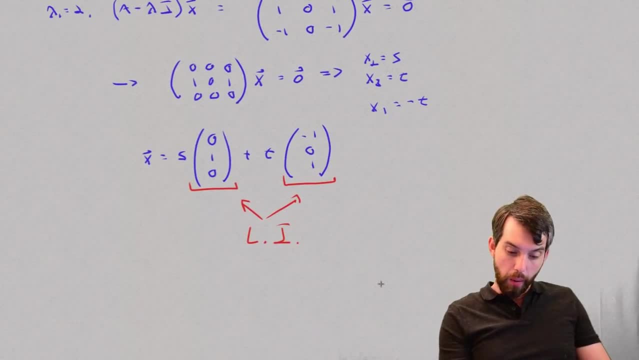 to that in a little bit. Now we had already input the lambda 1, equal to 2.. So for the next one let's do lambda 2, which I believe was equal to 1.. And so when I look at my a minus now, it's going to be lambda 2.. 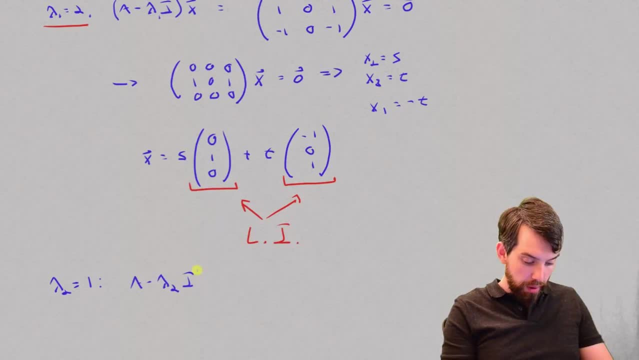 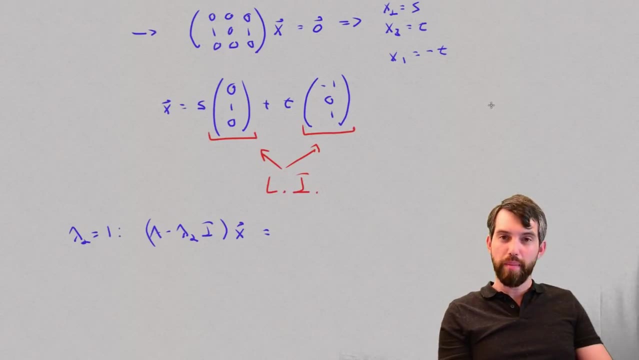 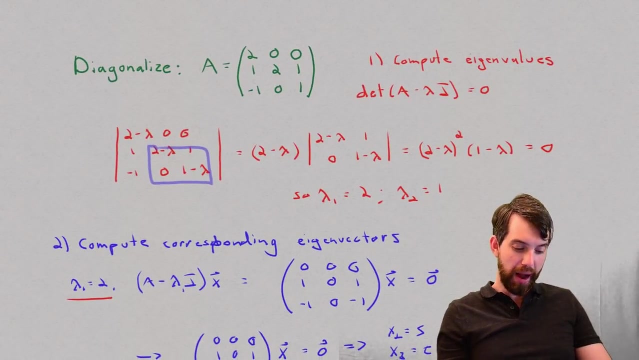 The previous one was lambda 1.. When I look at a minus lambda 2 times, i times the vector x. all right. well, I have to remember what my matrix A is before I subtract the 1s from the diagonal. So there it is: 2, 0, 0, 1, 2, 1, minus 1, 0, 1.. 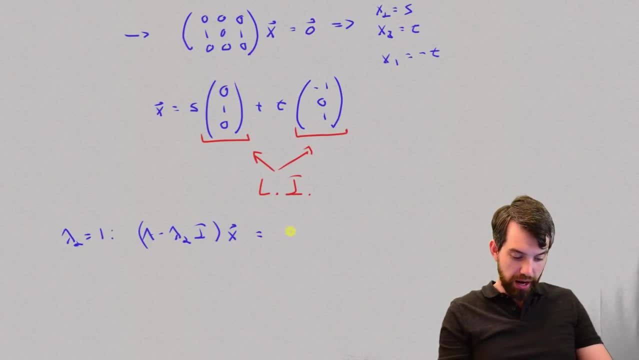 So I can subtract off the 1s all the way along the diagonal. So the 2, 0, 0 is going to go to a 1, 0, 0.. The 1, 2, 1 is going to go to a 1, 1, 1.. 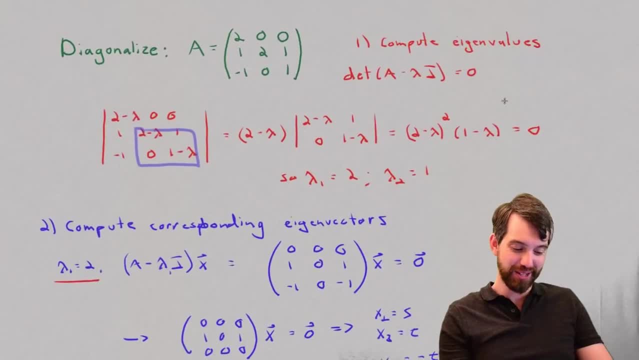 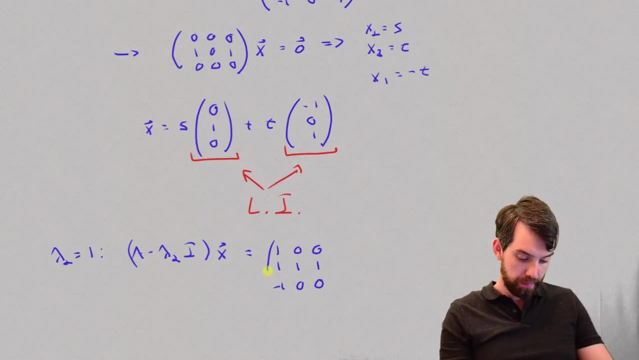 I've already forgotten the third one, So I'm going to subtract that The third row a minus 1, 0, 1.. And so I can put that in as minus 1, 0, 1, minus 1, another 0.. 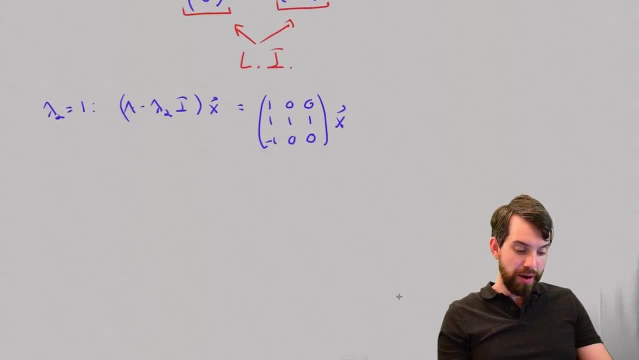 So I've got that matrix times x, And then what I want to do is do some reductions of this. I want to see what that's going to go to, So I will send that to 1, 0, 0.. I'll subtract off the first row from the second. 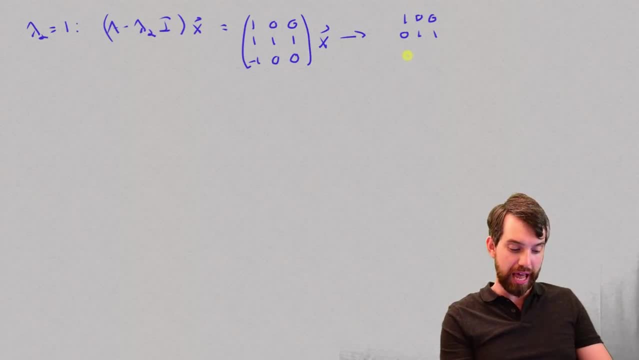 That gives me a 0, 1, 1.. Add the first and the third. That's going to give me a 0, 0, 0.. And I'm investigating: when is that equal to 0.. Well, we've got one free column here. 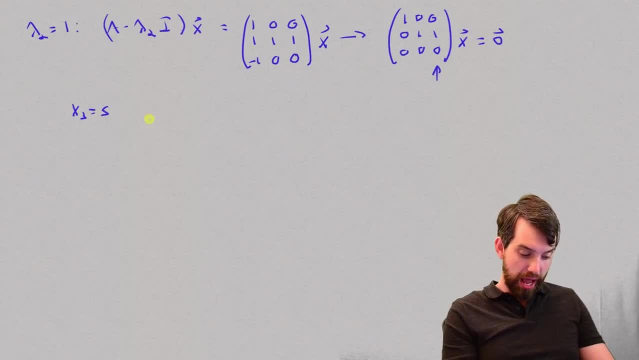 So I will set my x3 to be equal to s. I'm going to set my x2 to be equal to minus s, And that gives me that my x1, because it's the two 0s that has to be equal to 0. 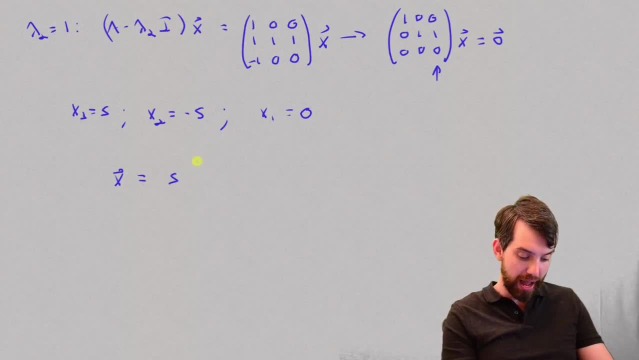 And so the standard way I'm going to write the vector x is this parameter: s. There's nothing in the x1.. There's a minus 1 times x1.. There's a minus 1 times x1.. There's a minus 1 times s in the x2.. 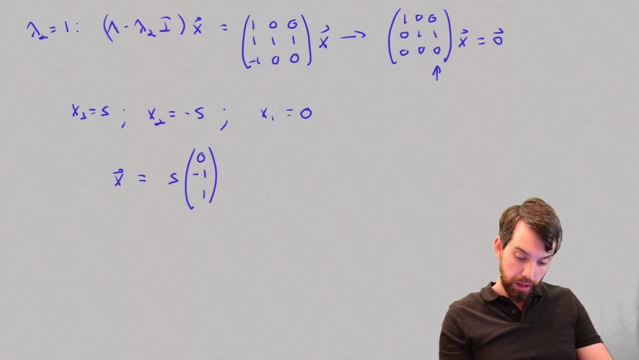 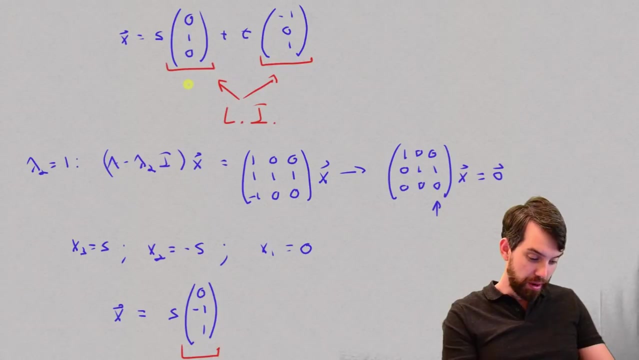 And there's a 1 in the x3. So what do I have? I have one eigenvector here. I'm going to call this v3.. Previously we'd seen that we had two other eigenvectors And they were going to be this v1 and this v2.. 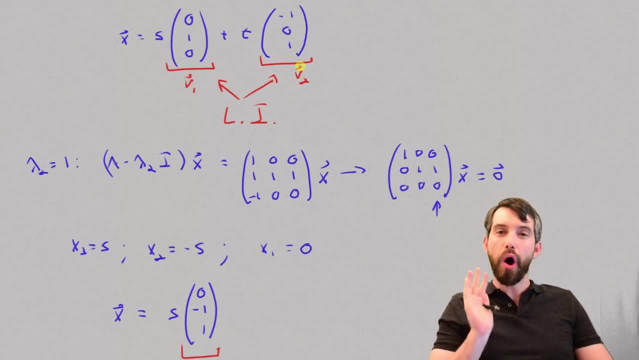 So I have one, two, three different eigenvectors, And they were all linearly independent. Why? Well, We've already argued that the two corresponding to that lambda 1 equal to 2, the two different eigenvectors we had there, those were linearly independent. 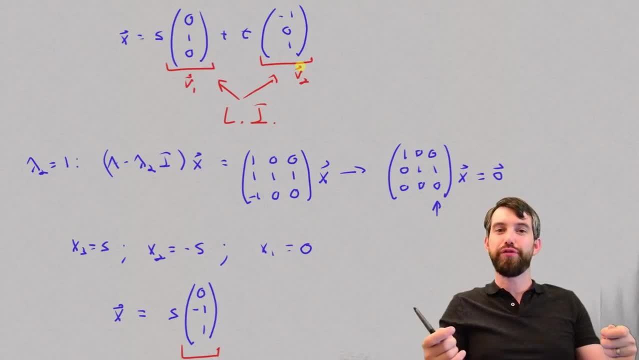 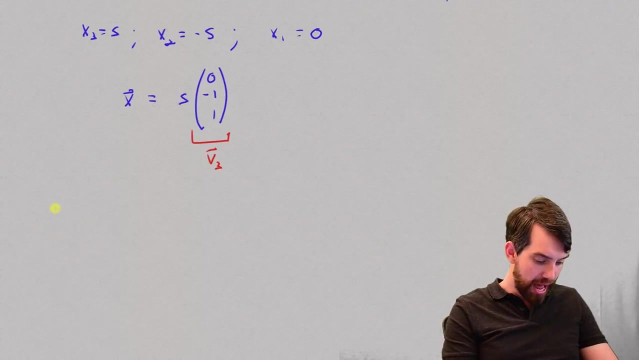 But we've also previously seen that the eigenvectors for different eigenvalues have to be linearly independent as well. So these three different, linearly independent eigenvectors are hanging around and I can put them into one matrix P. So this takes me now to my step 3.. And what I'm going to do here is create a matrix P. So this takes me now to my step 3.. And what I'm going to do here is create a matrix P, And it consists of the v1,, the v2, and the v3. 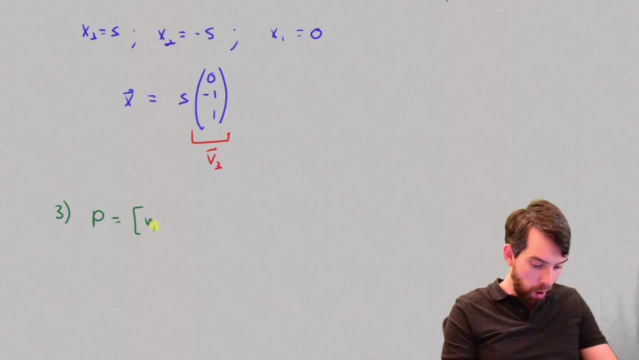 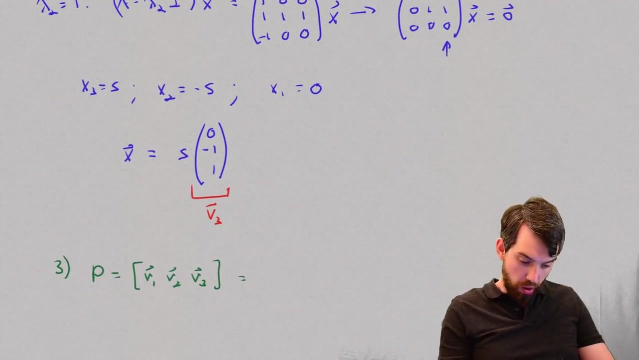 And it consists of the v1,, the v2, and the v3.. Which I have to scroll back up so I can see them. What's it going to be? 0, 1,, 0, and So I'm going to make a matrix: 0, 1,, 0, and. 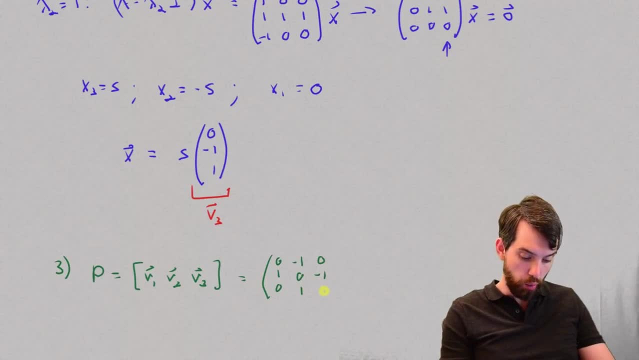 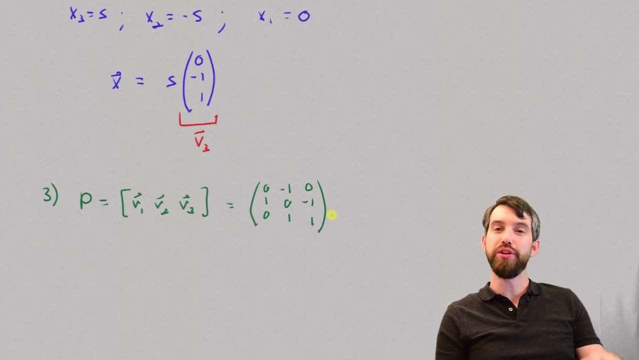 Those are my v1 and my v2.. And look, I've got a third one here, Minus 1, 1.. 0, 1, 0,. and Now, if you're unsure, you could do a quick check at this point and verify by doing row. 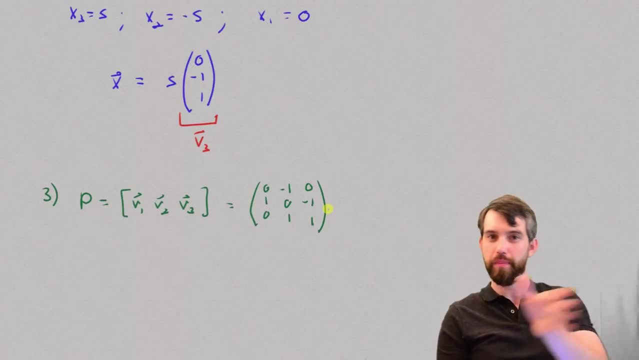 operations, that this matrix was indeed invertible, that there was a pivot in every row and every column. And if that wasn't the case, then it is either not going to be an invertible matrix- as in the eigenvalues you don't get a full set of n linearly independent ones- or perhaps 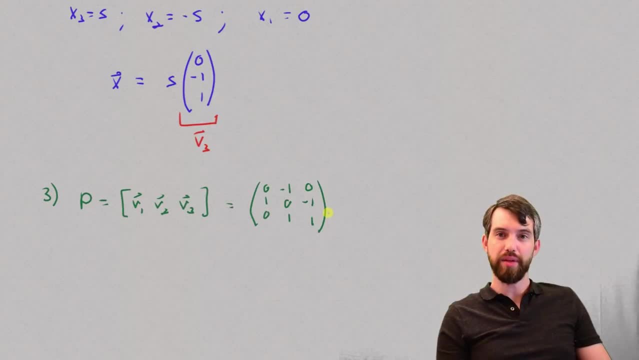 you've made some mistake in your computation. We've got this p here and there's going to be a p inverse. I'm not going to bother computing it, but we could do it. And then, finally, what's the d matrix going to be?